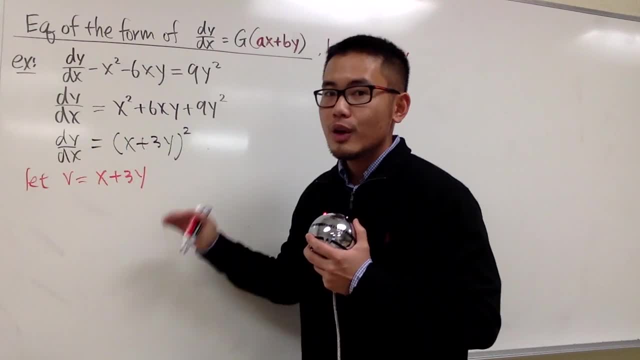 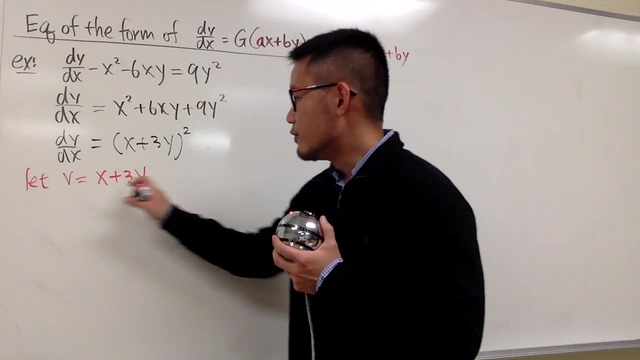 We have to take this differential equation, which now is in terms of x and y, only We have to change that into a differential equation to be in terms of x and v. So, with that being said, I'm going to differentiate both sides. 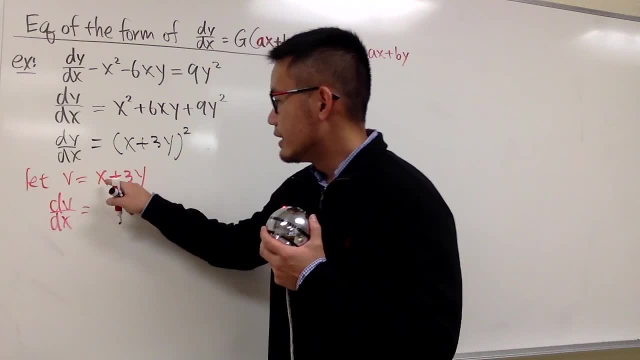 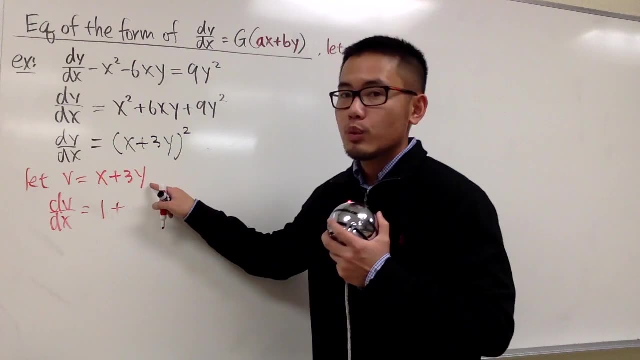 So we have dv, dx, and this will be the derivative of x with respect to x, is just 1.. And then we add it with the derivative of 3y with respect to x. Well, you know, y is a function of x. 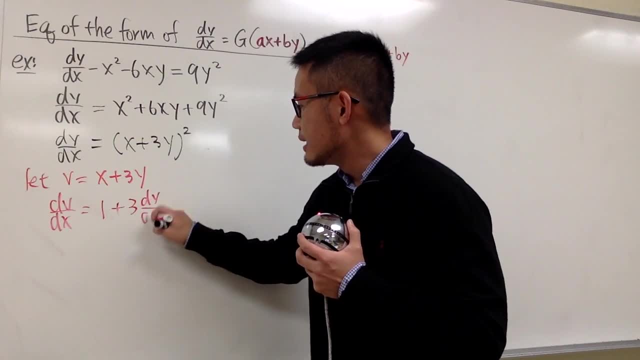 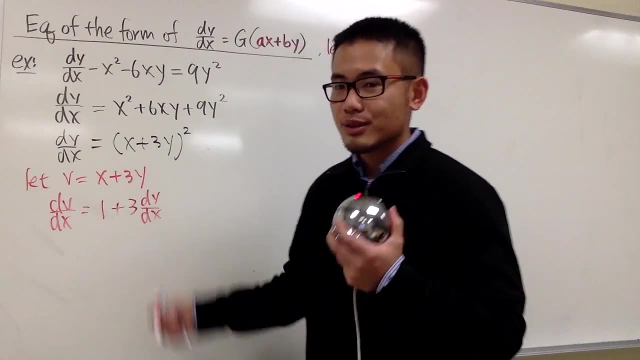 So this right here will be 3dy And this will be 3dx. like this: I showed technical install for the dy dx so I can plug in right. So let's go ahead and do that. Let's isolate the dy dx right here. 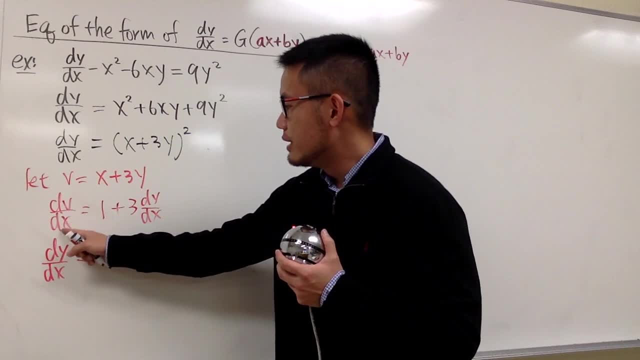 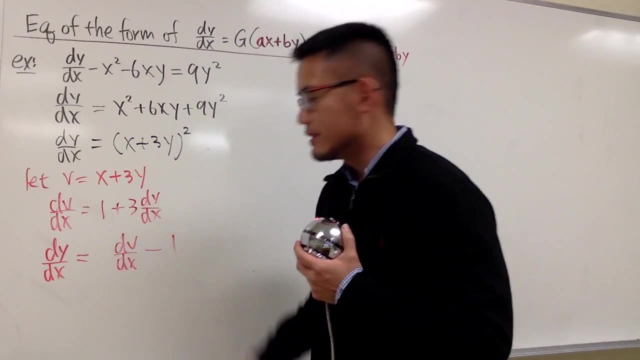 And let's do a few things in our head First. I will have to put this and that right, And I want a minus 1, so we will have dv dx minus 1, like this. However, I should have this 3 right here, but we have to divide everything by 3.. 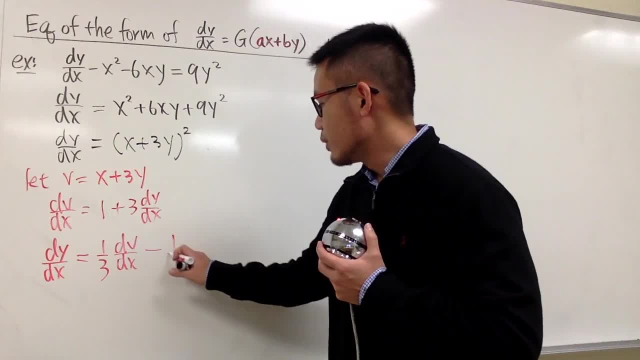 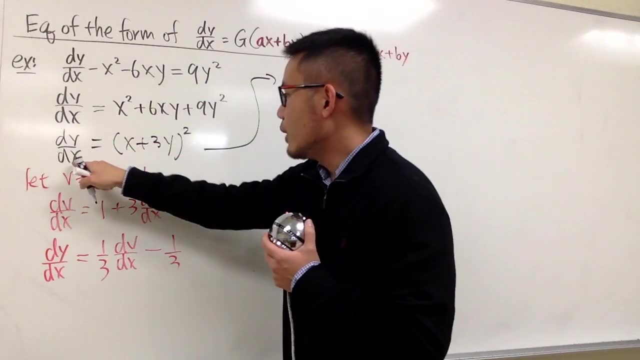 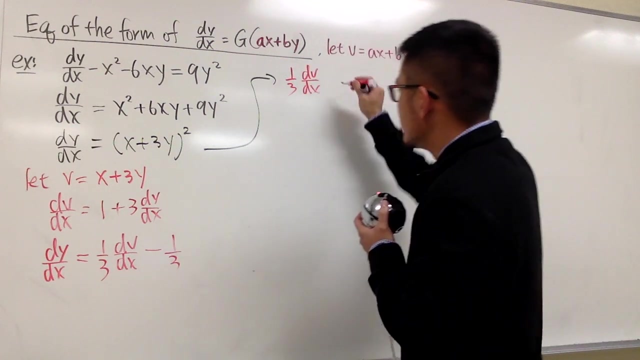 So we will have the 1 third And then minus 1 over 3 instead, like this: okay, All right, so we'll write this For the dy dx to be that we have 1 third dv dx minus 1 third. 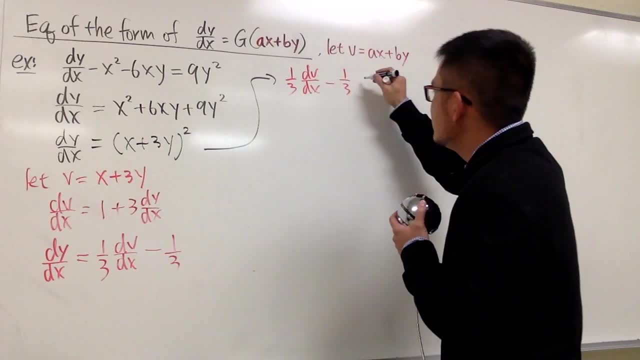 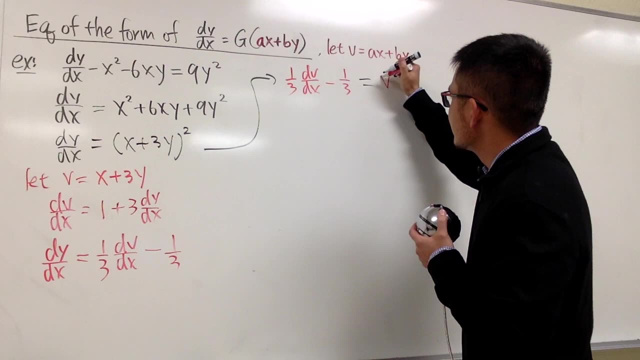 The whole thing. now, this right here represents the dy dx And this is equal to the input. here is the phi. So we have: this is equal to phi and we square that. okay, And usually we don't like. We don't like fractions in the equation, so let's multiply everything by 3.. 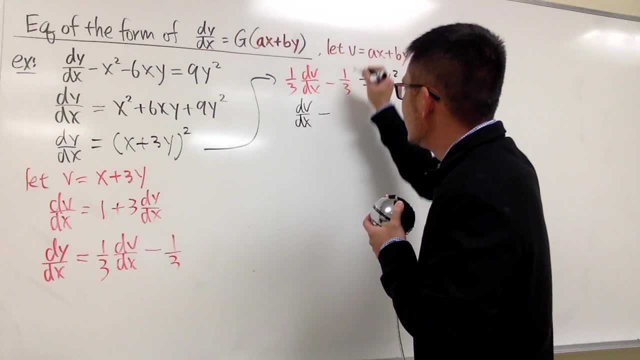 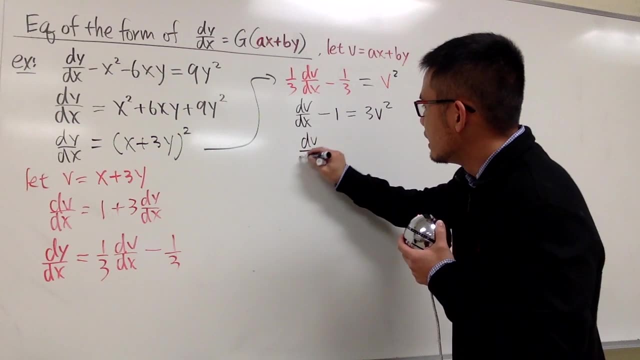 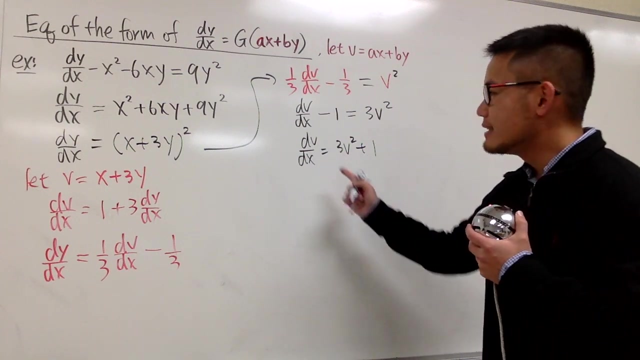 Therefore, we'll end up with dv dx minus 1, and this will give us 3v squared. And add the 1 on both sides, you'll see we have dv dx equals to 3v squared plus 1.. And now you see, we can just divide 3v squared on both sides and we can multiply dx on both sides, right? 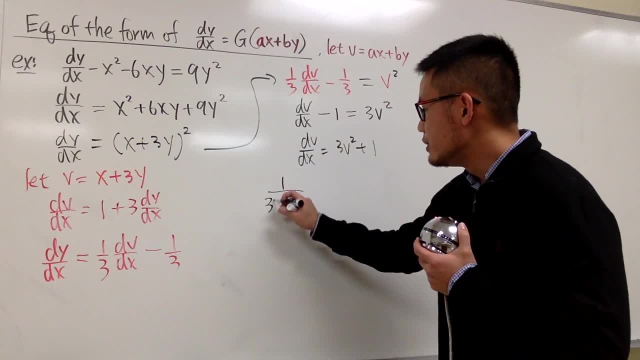 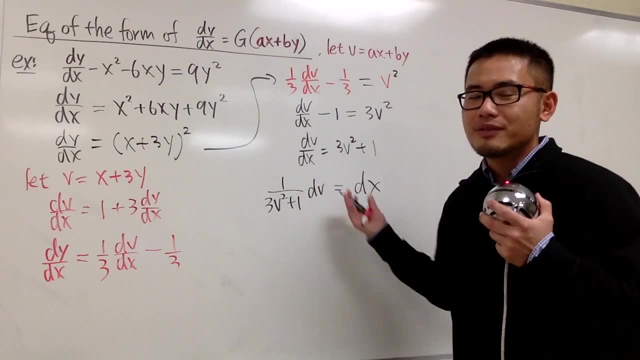 So on the left-hand side we'll write it as 1 over 3v squared plus 1 dv, and this is equal to dv- dx and we just separate the variables. All the v's and dv's are together and we have the dx right here. 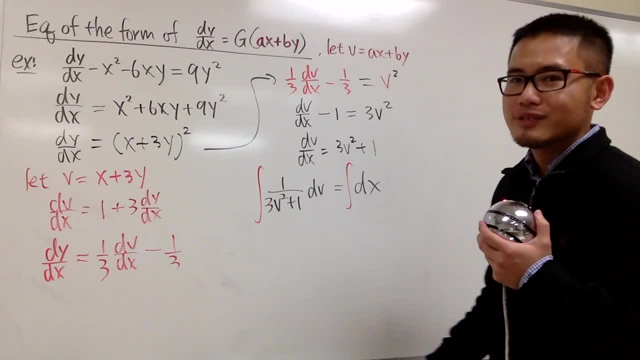 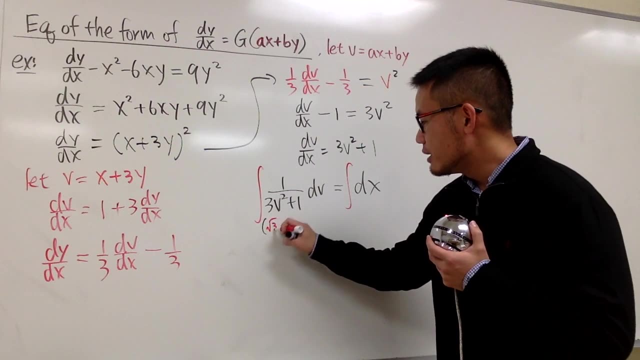 And, with that being said, we can go ahead and integrate both sides. To integrate this, I'm going to look at 3v squared- as parenthesis- square root of 3 times v, and then square, and then we still have the plus 1 after that, right. 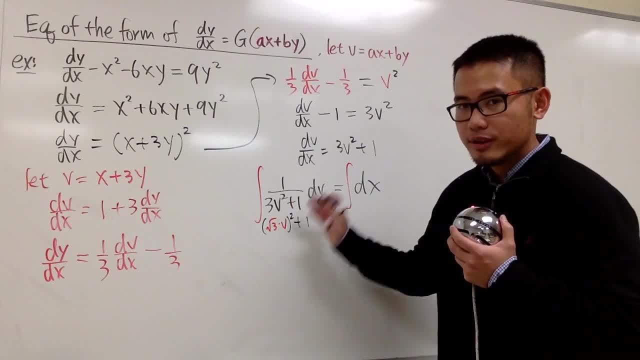 1 over something squared plus 1 for the integral. we know it's going to be inverse tangent, So let's put that there: 1 over something squared plus 1 for the integral. we know it's going to be inverse tangent, So let's put that there. 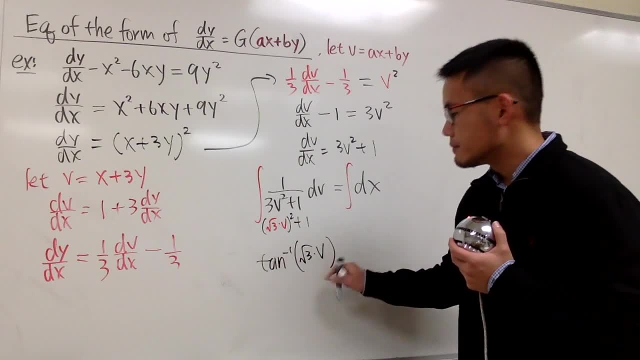 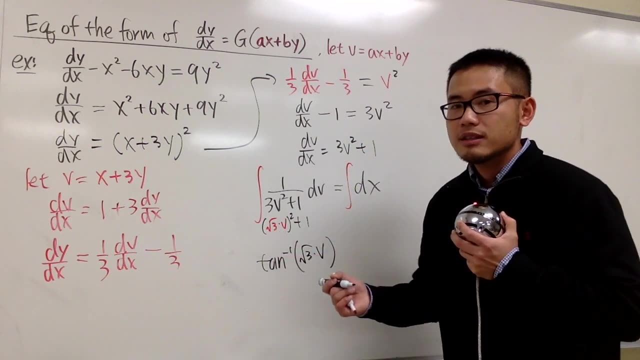 1 over something squared plus 1 for the integral. we know it's going to be inverse tangent, So let's put that there And the input is square root of 3 times v. But we're doing integral, right. So the derivative of this square root of 3 times v is square root of 3.. 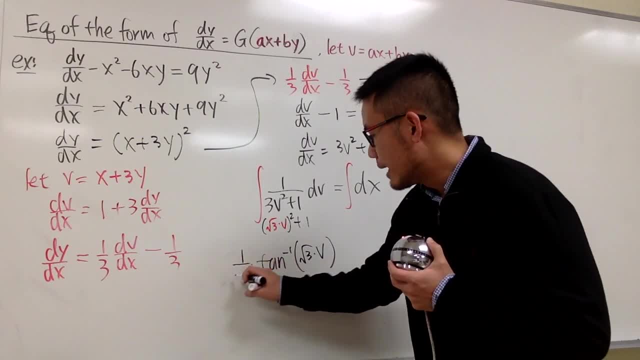 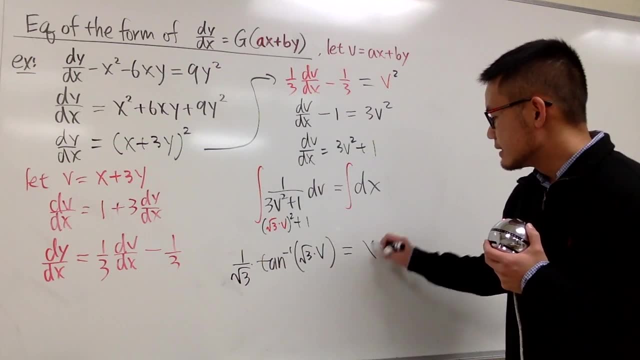 So we have to divide it by square root of 3, which is the same as saying: multiply by 1 over square root of 3, like this: That's the integral for that, And this is equal to x, And we put down the constant on the right-hand side. 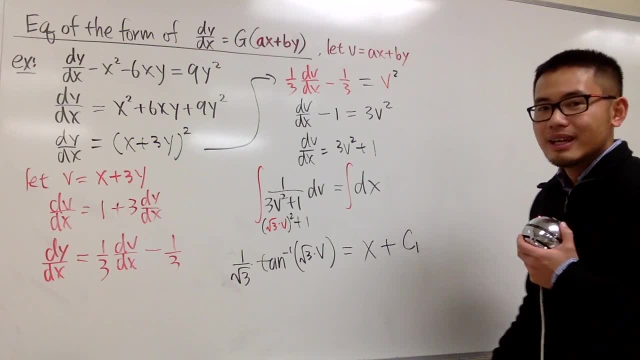 So let me put down plus c and let me just say c1.. Because I want to solve for the 3.. And this is equal to x, And we put down the constant on the right-hand side. So let me put down plus c and let me just say c1.. 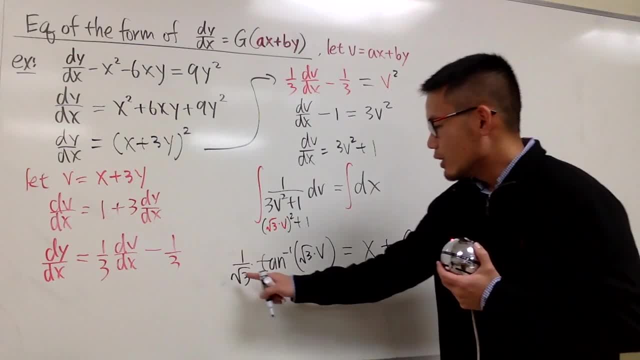 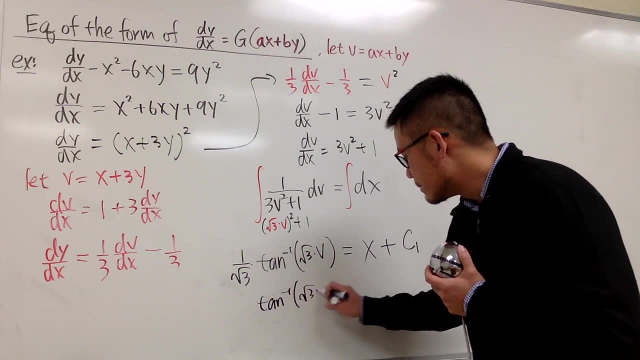 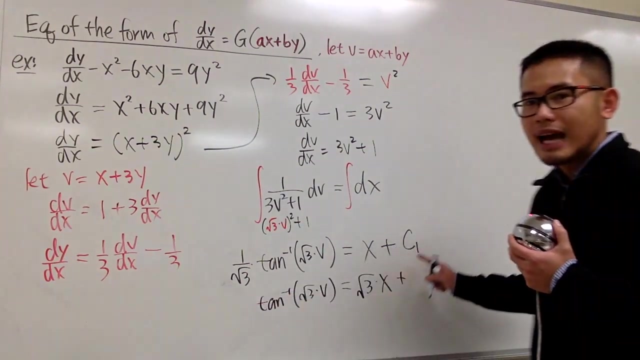 So for the 3, and then at the end I will get the y. So let's multiply everything by square root of 3.. So we will have inverse tangent of square root of 3 times v, And this is going to be square root of 3 times x plus square root of 3 times c1.. 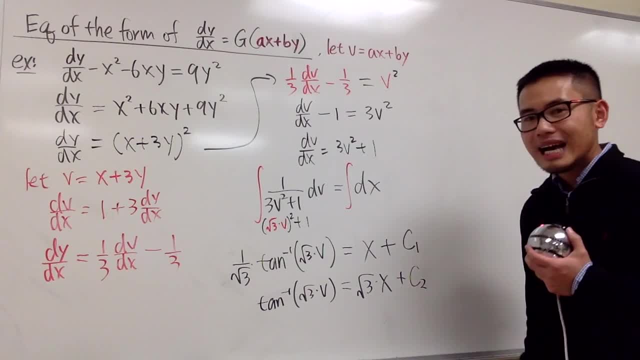 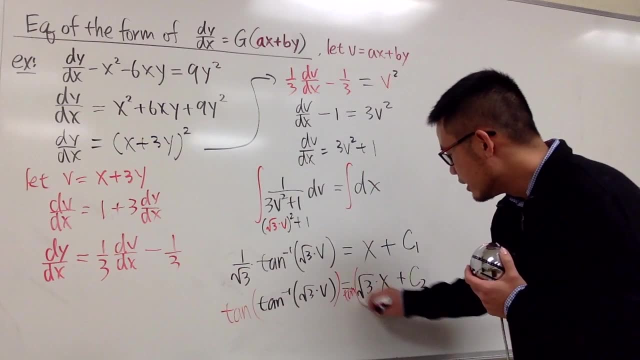 It's just another constant. so let's put down plus c2. And that's what we have, right? And now let's take the original tangent on both sides. So let me just show you guys the work. right here We take the original tangent. 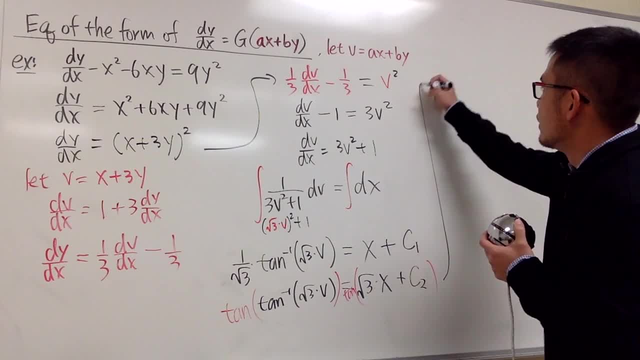 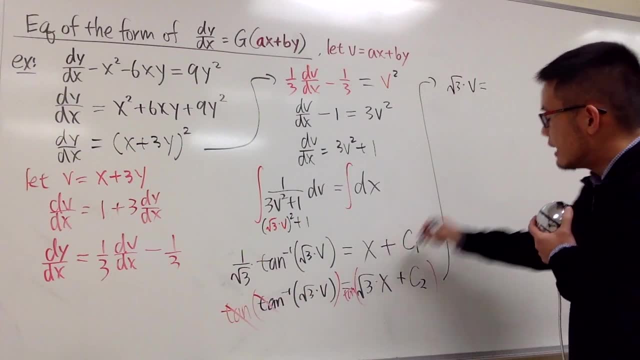 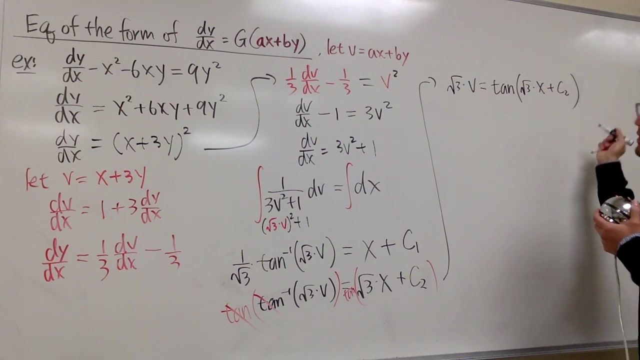 And be sure, both of this are in the original tangent And now we will have this and that being cancelled here. Square root of 3 times v equals to tangent of square root of 3 times x plus c2.. Like this: 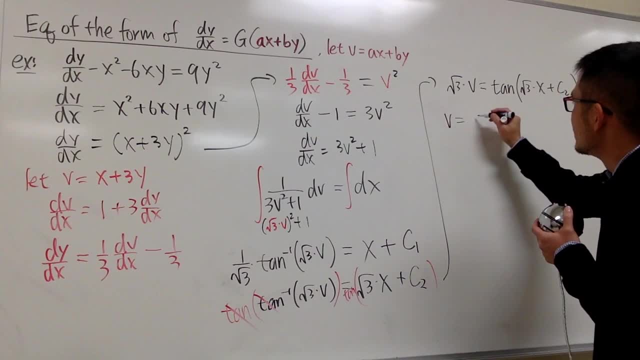 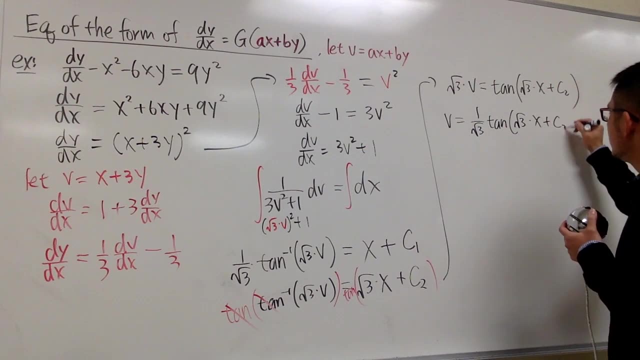 And of course divide by square root of 3 on both sides, So we get v equals to 1 over square root of 3. Regular tangent. and then square root of 3 times x plus c2.. Like that, Okay, we got the v by itself.